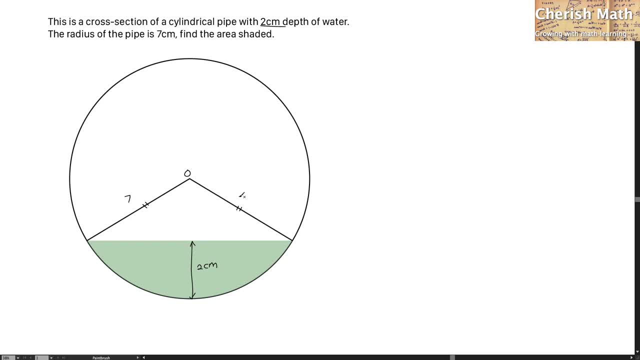 The radius of the pipe is given as 7 cm, And now, if I connect from the center to this line, I'm going to find that the height on the white space here is at 5 cm, simply because I'm going to use 7 cm as the radius of the circle. 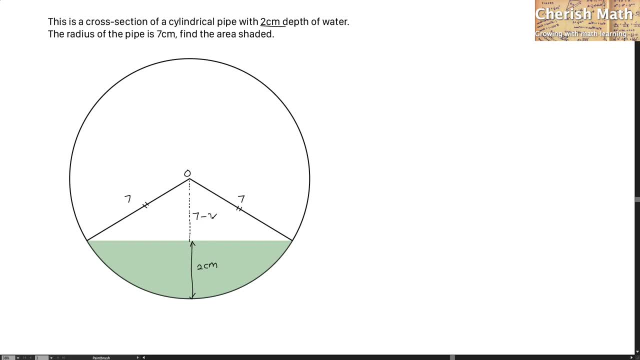 minus the depth of the water, which is at 2 cm, and I get 5 cm, And for the dotted line here it's going to form a right angle with the level of the water And I have to work out what is this angle that I'm going to name as theta. 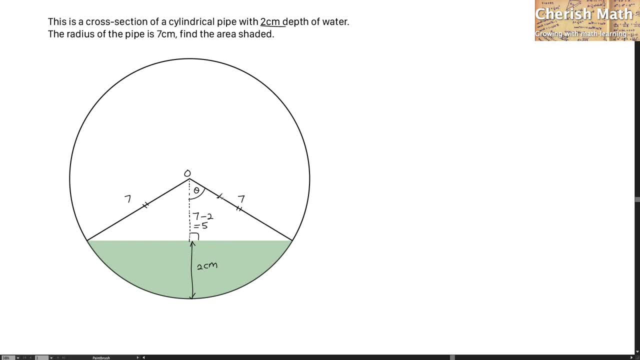 By referring to this right triangle. I'm going to find the value of the theta by using cos theta adjacent of the cos theta. So the theta is 5 and the hypo is going to be 7.. So the theta I can find it out by using the calculator, which is 44.4 degrees. 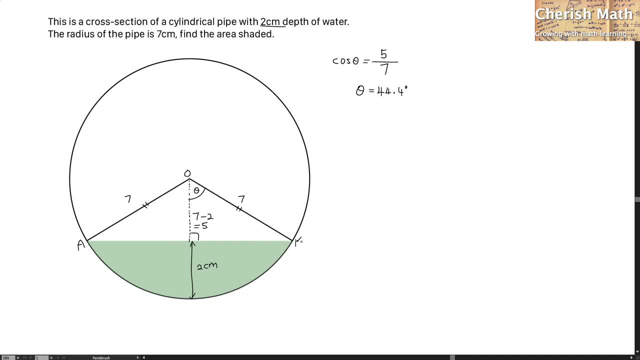 I'm going to label the part here as A and this part as the B. Now, the angle for A O B is twice the value of theta, simply because this triangle that is located on the left hand side and this triangle that is located on the right hand side are both identical. 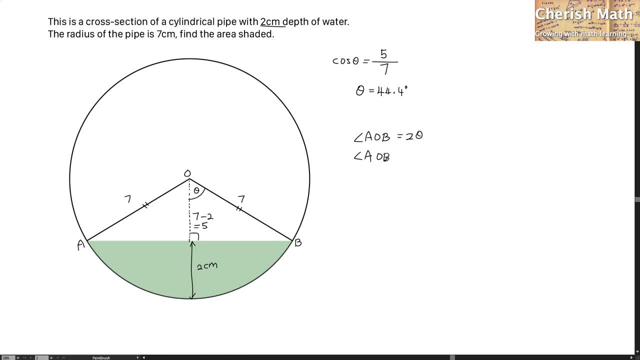 So now the value of the A O B turns to be 2 multiplied by 44.4 degrees, and the value of A O B is 88.8 degrees. And now I'm trying to find what is the shaded area here in green color by using